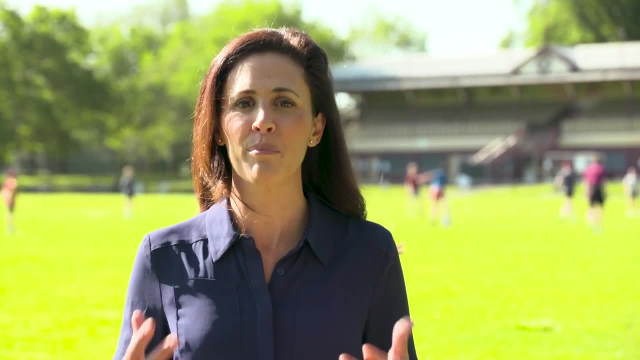 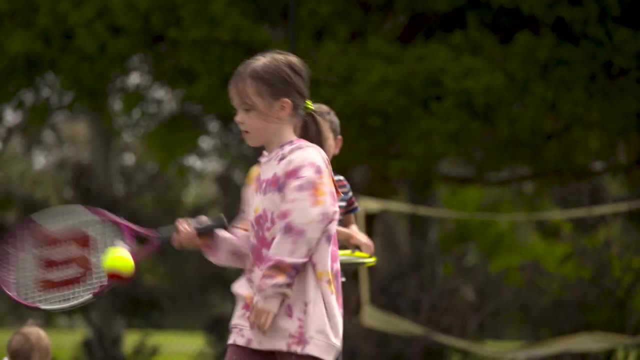 Community. sport and other organised physical activity is one of the best ways for kids to keep physically and mentally well. It was great to learn that almost all parents recognise that sport and organised physical activity lifts their child's physical and mental well-being. One in three say 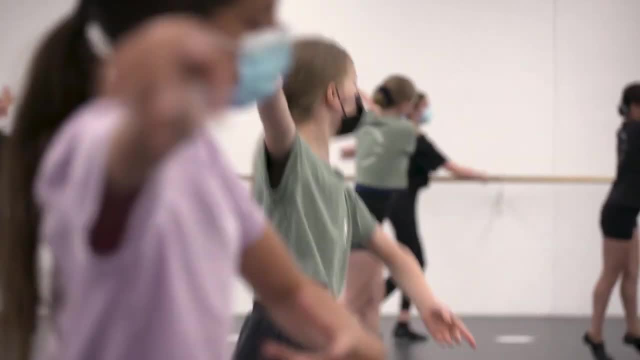 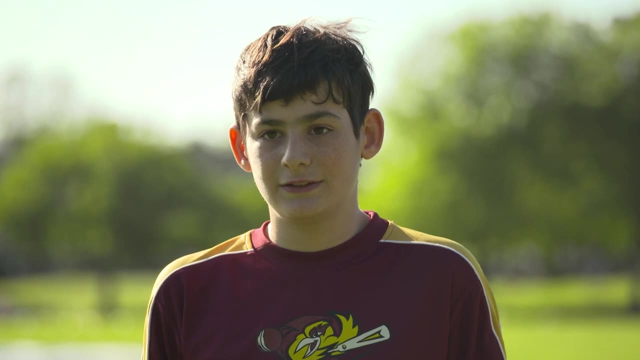 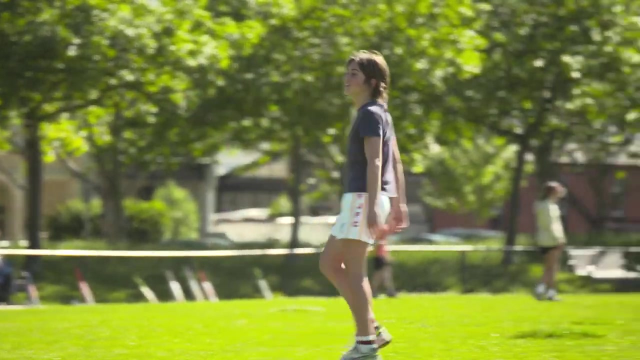 it's even more important now than before the pandemic. I get to bond with people that like the same thing as me and like it's very relaxing. I just love, you know, being out in the sun playing with maids, having a good time. I know some people think it's about winning. honestly, I'm one of those. 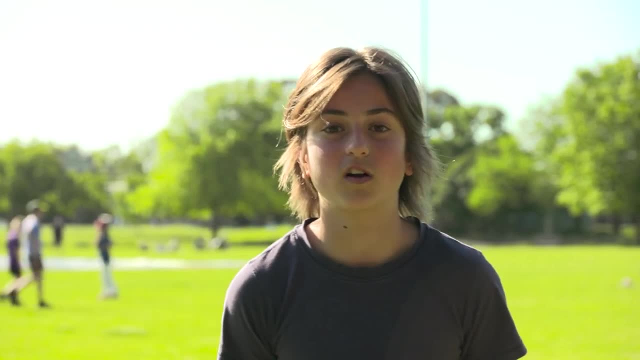 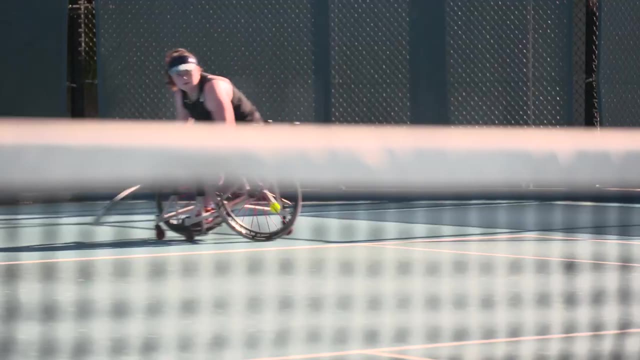 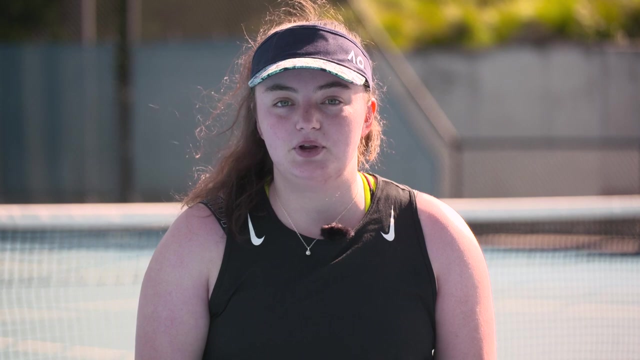 people, but a lot of the time I just like playing sport for the fun of it all. Definitely it's a lot better in person. I think it distracts from anything that I've done that day if I've not had a great day. it's just such a good boost and it, you know, makes you feel really good. 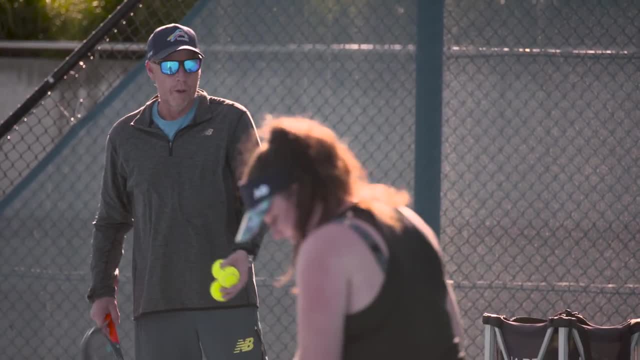 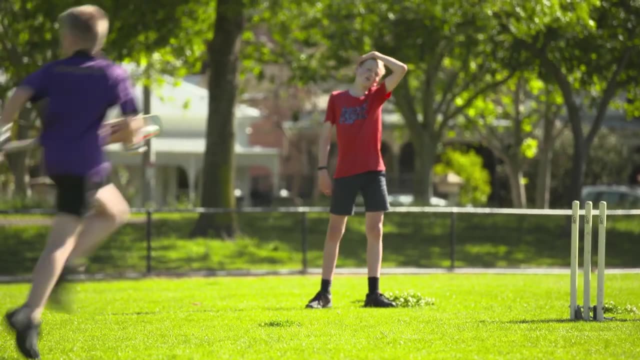 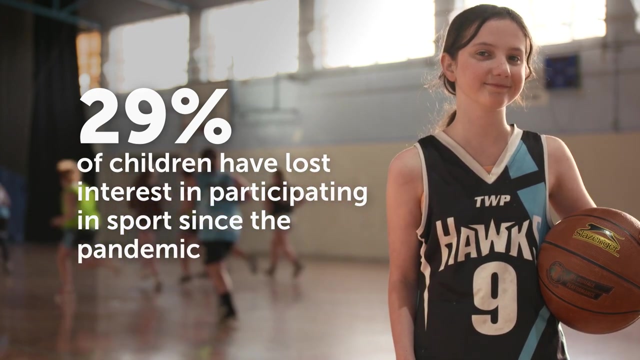 and, like you've gotten out and done something, and so I think it really pushes me to be better. Healthy habits can be hard to make and easy to break Around. a third of kids say they have lost interest, are too busy or no longer feel fit enough to get back into community, sport or 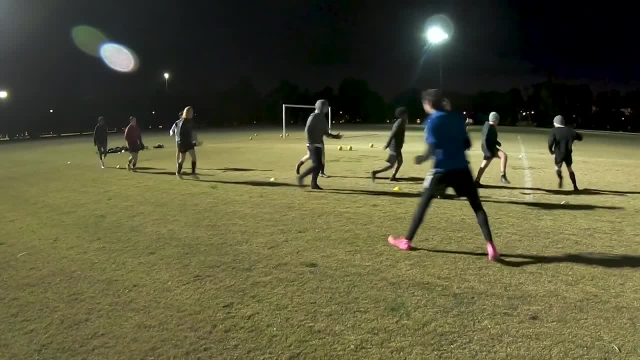 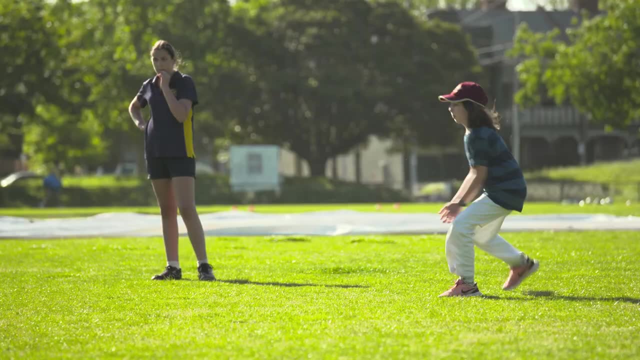 other organised physical activity. The earlier you can get back into sport and build a routine, the easier it will be. If your child is still feeling unsure about getting back in physical activity. you can get back into sport and build a routine, the easier it will be. 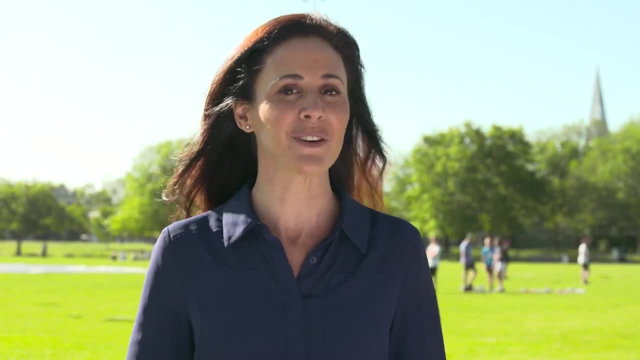 If your child is still feeling unsure about getting back in physical activity, you can get back in involved in community sport. We've got some great tips from the experts. Well, if you feel like you've lost touch with your friends, all you have to do is just go to. 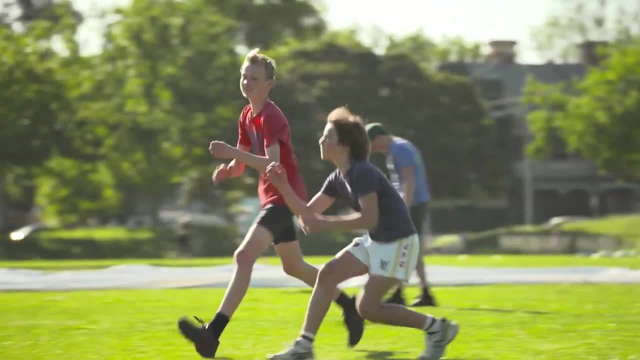 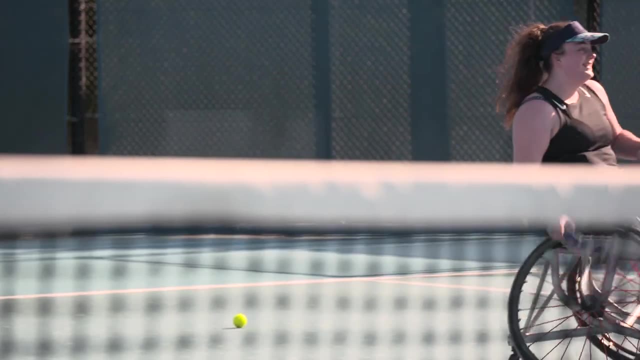 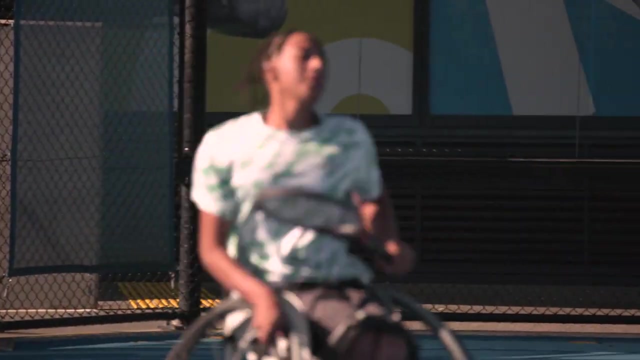 the trainings and you'll see them again and you can get back in touch. If you're feeling unfit, go back to the trainings. you can get fit again. The first time we got back on court after lockdown I was hitting terribly, but I think that that's something that if you have a good group of people around you and if you 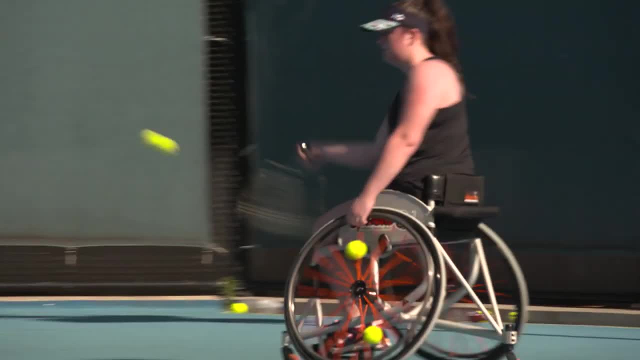 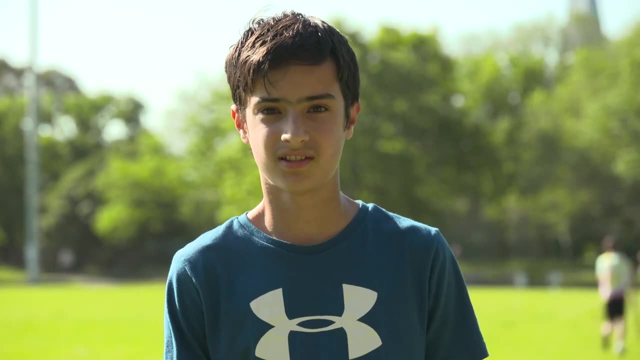 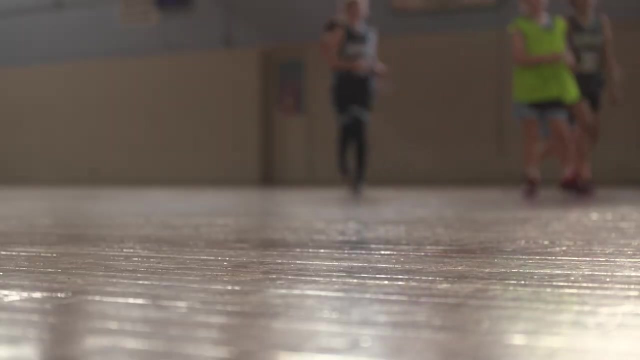 have the love for the sport, then you'll forget about that as soon as you get back on. It's hard at first, but you do make friends and you do get better. Just do it, because there's so many other people in that situation, While one in three parents are worried about their child being exposed to COVID playing sport.